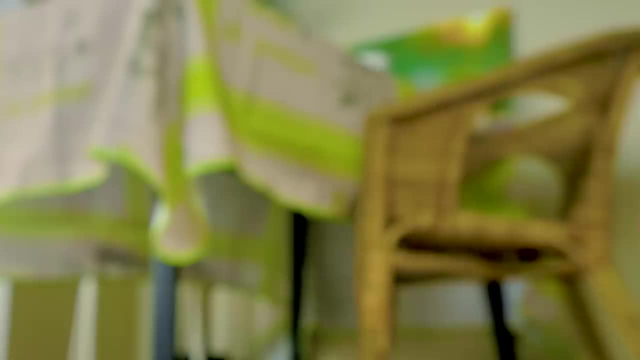 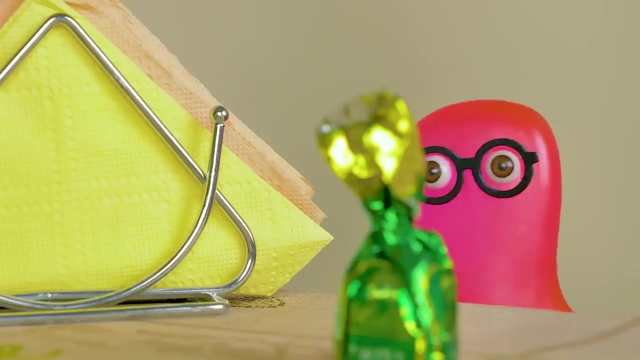 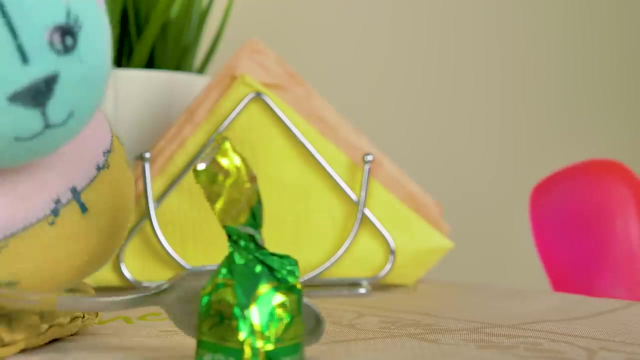 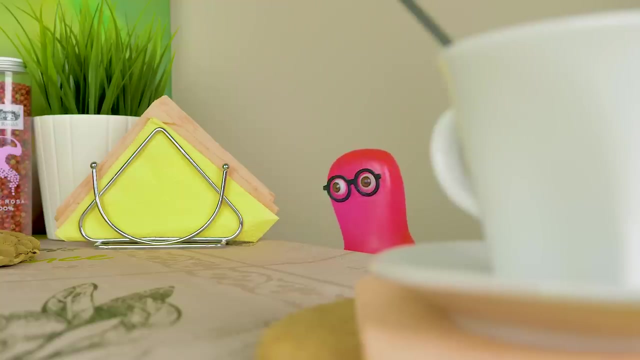 Nope, nothing to do here. Ugh, Oh chocolate, will you cheer me up? Huh, What's that? Huh, Maybe I'm uh hearing things. Uh, where's the chocolate? Where did it go? 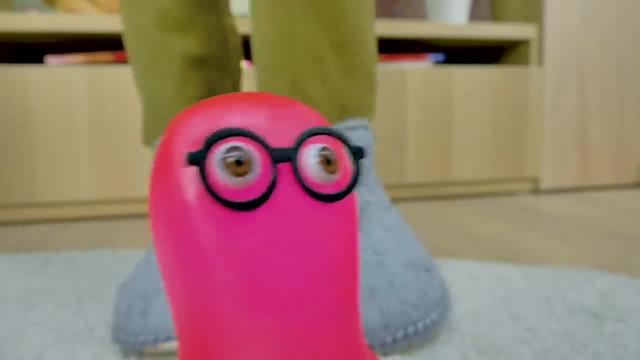 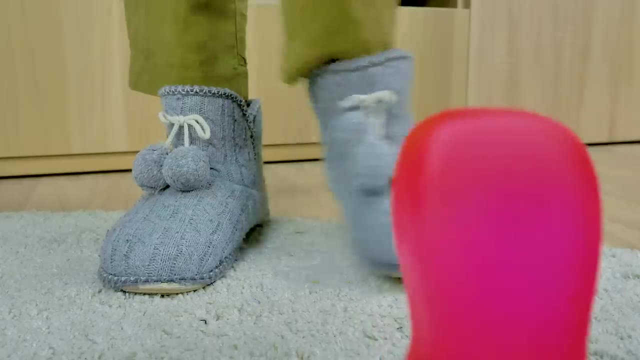 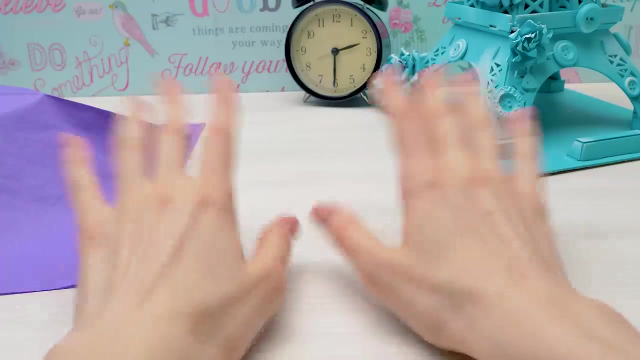 Sammy, are you here? Susie, You're back. I've been going crazy with boredom. I even started to see things You did. We need to start entertaining you then Come on. Hi guys, Looks like I have a difficult task ahead of me. 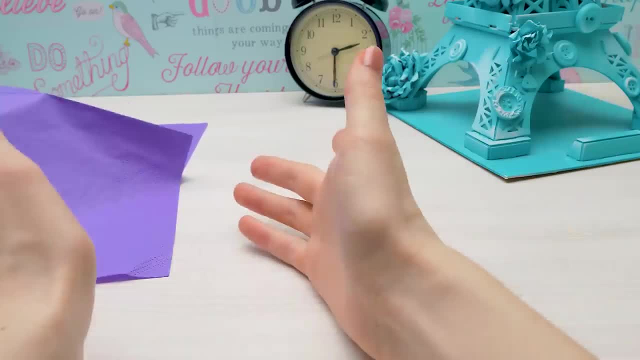 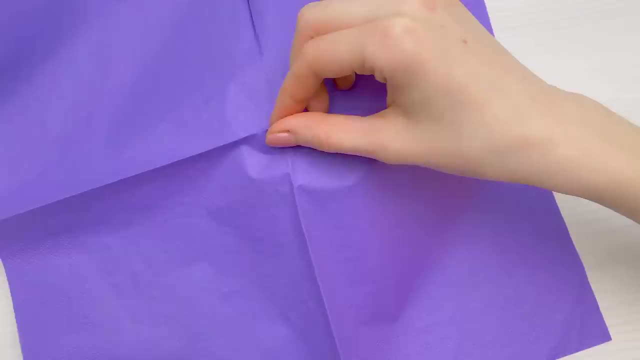 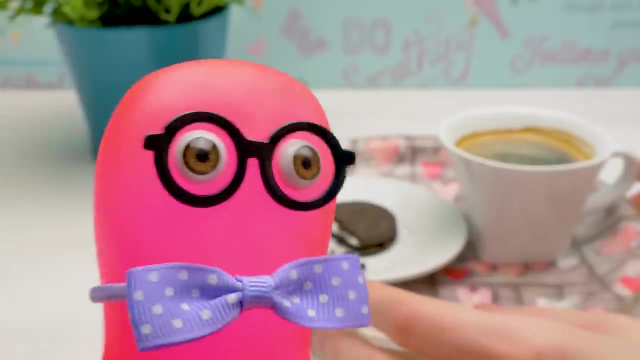 To entertain a bored Sam. Oh, what's this? I? I put it together for you. I thought you'd come home and see the surprise. Oh, Sammy, This is wonderful. Coffee, cold and a cookie half-eaten. Well, I prepared it a long time ago. 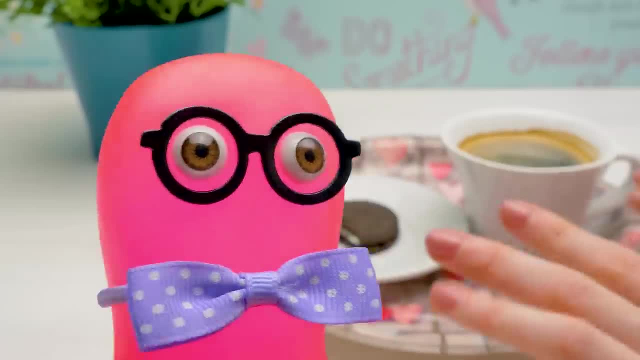 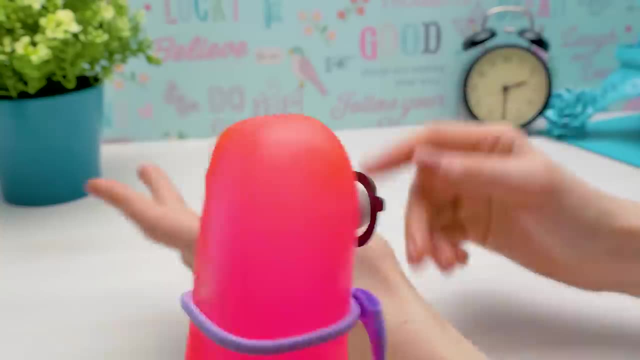 I didn't know you'd get back so late. That's why it changed in quality. Well, thank you for caring anyway. So how are you going to entertain me With all kinds of tricks? Tricks- Are you going to take a bunny out of a hat? 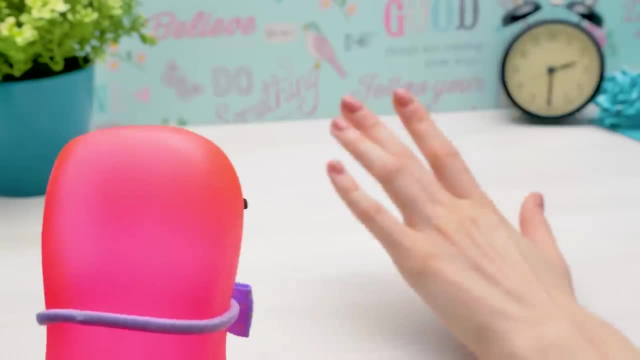 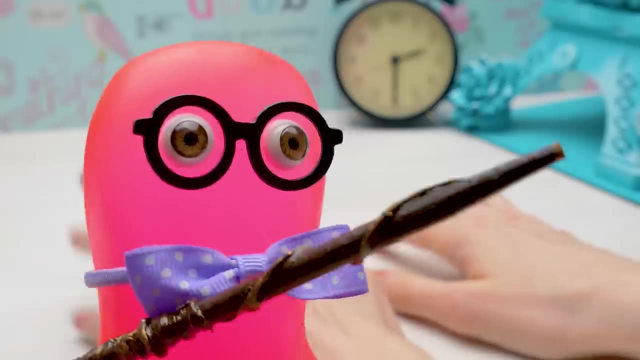 No, no, bunny out of hats, But it'll still be interesting, I promise Let's get started Here. What do I need? a wand for Sammy? Well, how are you going to do magic tricks With my hands, Sammy hands? 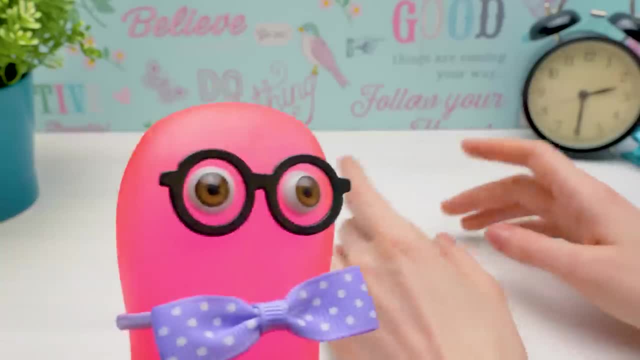 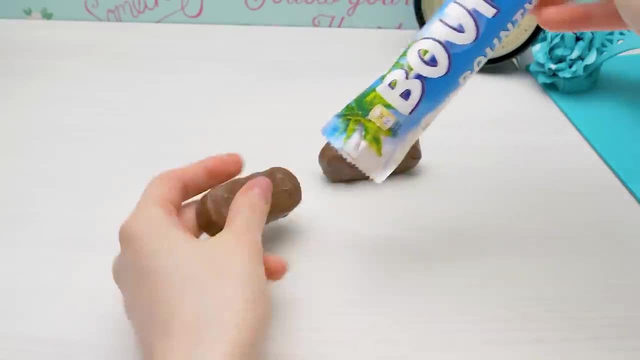 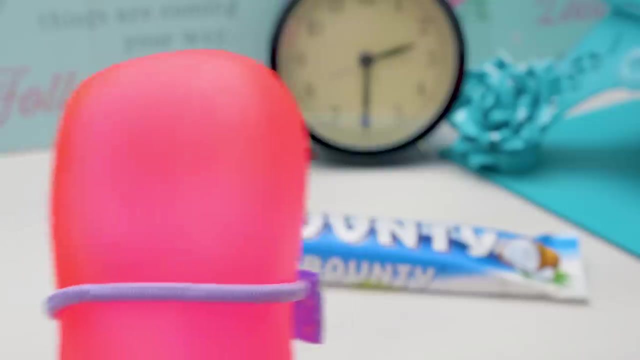 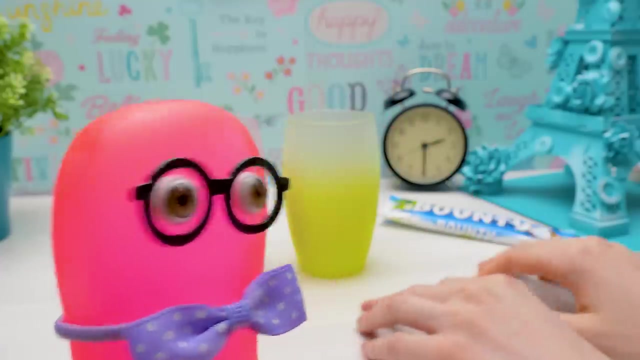 Well, alright, I'm watching closely. You better go and fetch me two glasses, Fine, And meanwhile, Here are your glasses. Thanks, What is this? What is this chocolate wrapper doing here? I need it for the trick, And where's the chocolate bar? 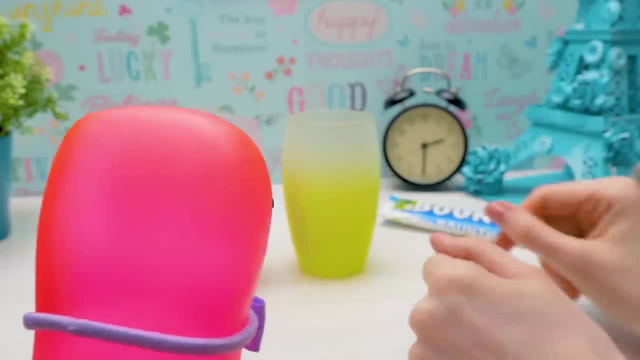 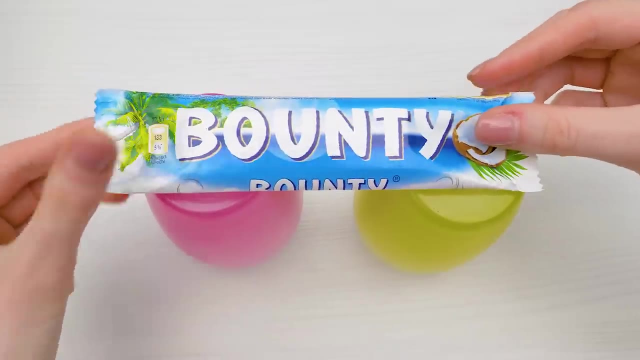 Gone. Uh Look, I'm going to show you the trick now. I'll take the glasses and place them like this, Then I'll place the wrapper on top of them, And now I'll remove one glass, But the wrapper will fall. 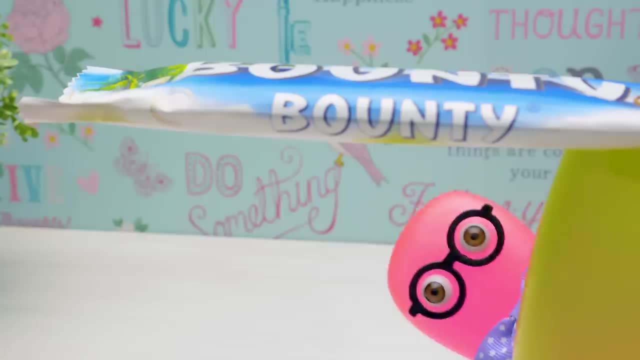 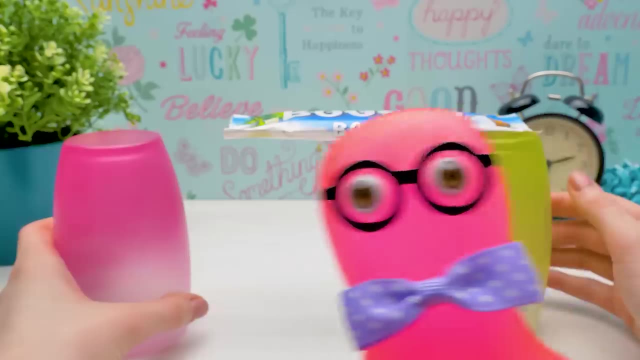 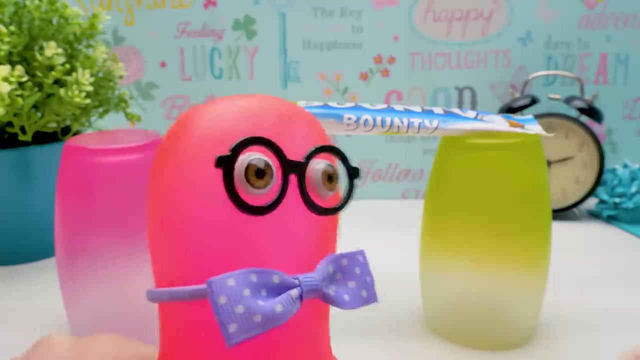 Look, How is that even possible? A wrapper can't just hang in the air, It's a trick, Magic. Oh, there has to be a secret to it. I'll tell you later. okay, Hey guys. Sue's left for the moment, so I'll show you a trick as well. 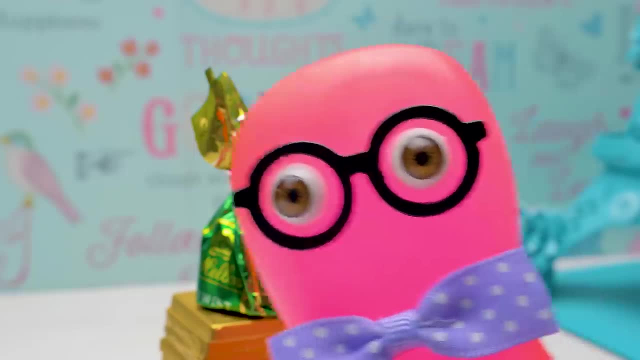 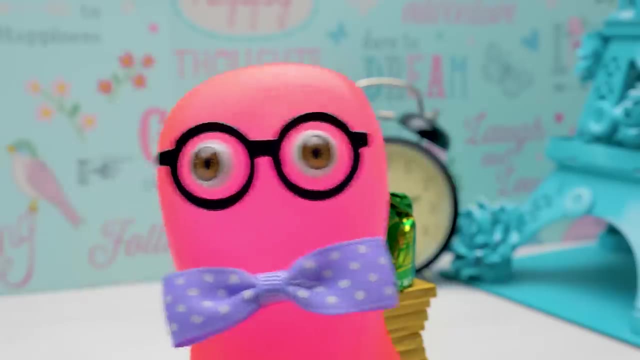 Here's a chocolate, See. And now poof, It's gone. Now you see it. Now you don't There? Only I can't reveal the secret behind it. It's an old trick. It's been passed down from one slime to another since ancient times. 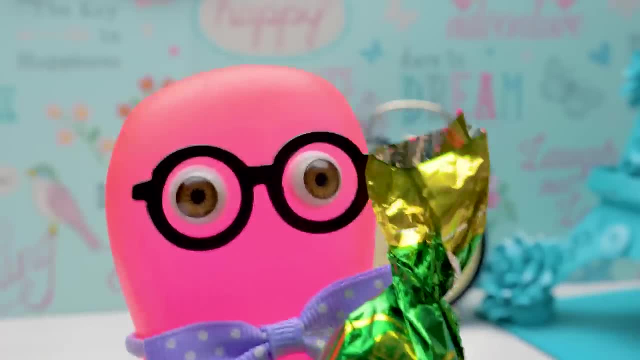 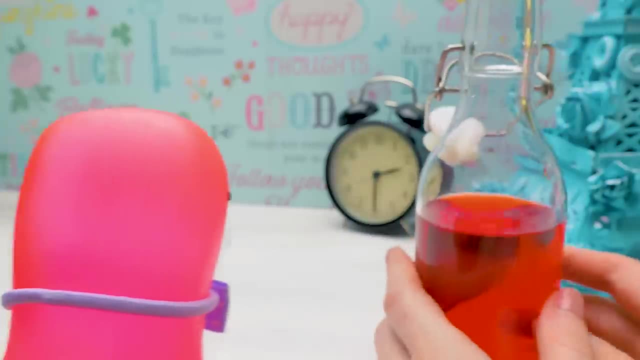 By the way, do you know any cool tricks? Write in the comments and I'll give them a try. Sammy, are you thirsty? Of course I am. Ah, then you'll like this trick. I hope you're not going to just pour the juice over me. 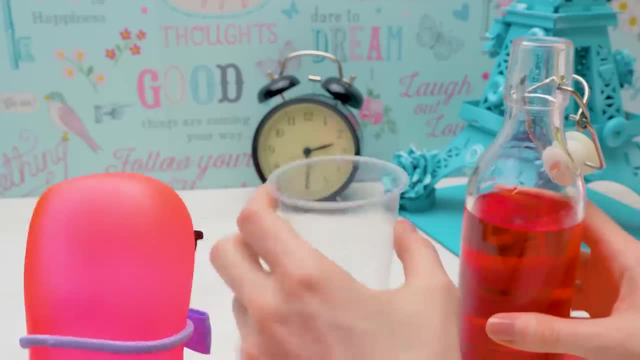 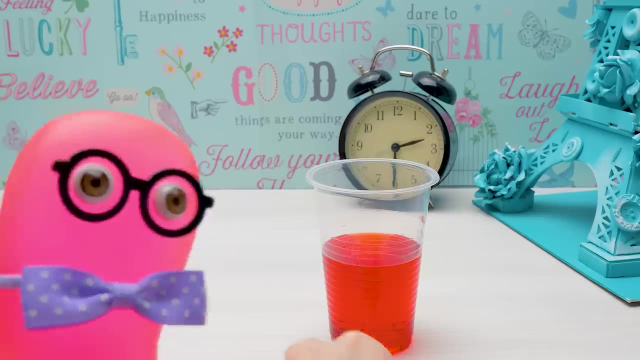 A juice shower sounds interesting, but No, no, I'm not, Don't worry. Then what are you going to do? Turn a half-empty cup of juice into a full one? Not quite. I'll take another cup. There's a bit of juice on the bottom. 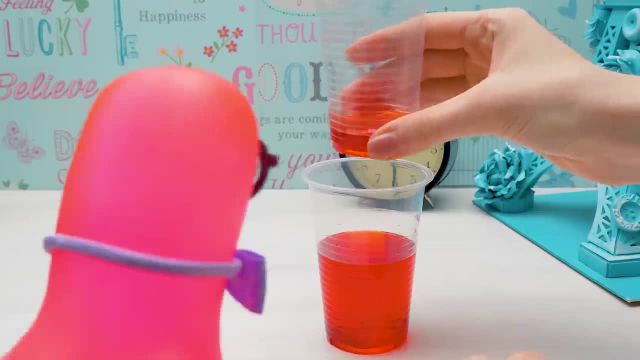 Oh, careful, you're going to drop it. Whoa, You dropped it Not to worry, And there's more juice in there now. There really is, But how? How did it seep through the bottom? I don't understand. 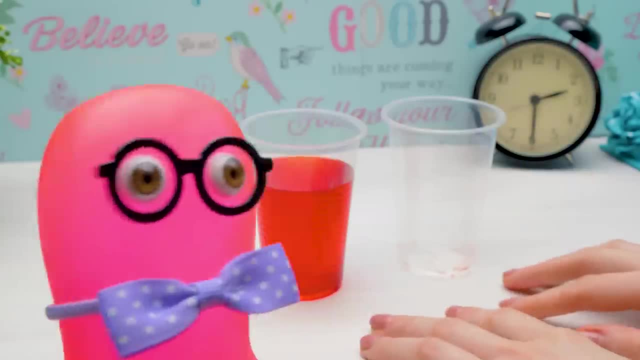 It's magic. I should check the juice. You might have ruined it with your tricks. Oh no, no, Sammy, I'll pour you some fresh juice. Hmm, Alright, I'll pour you some fresh juice. Oh Oh, I'm sorry. 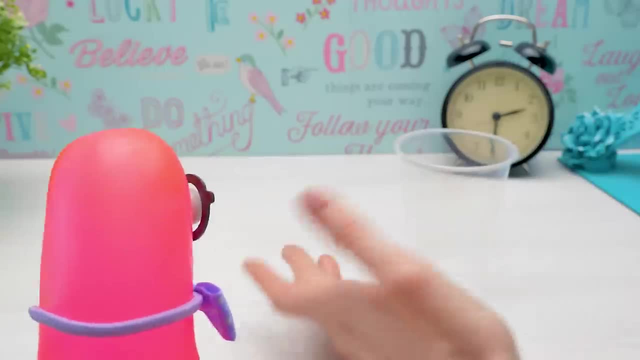 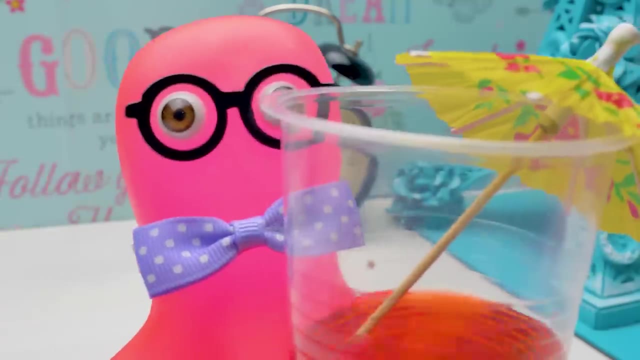 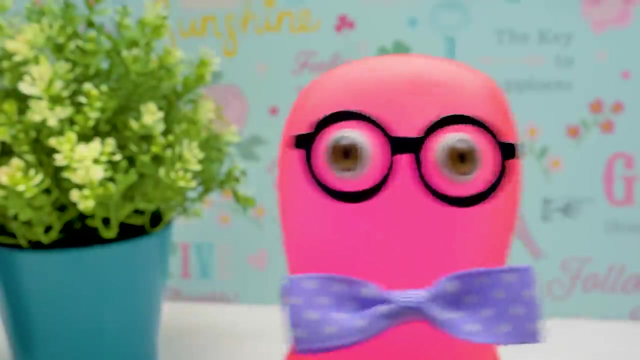 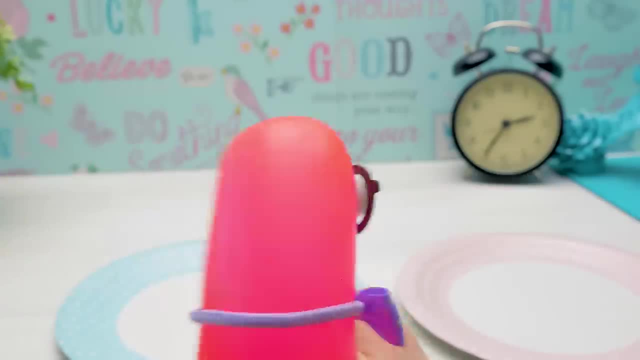 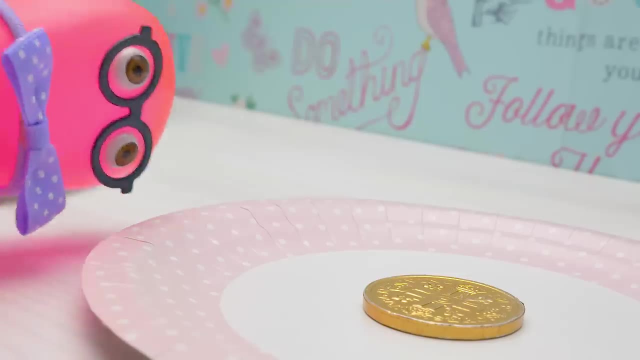 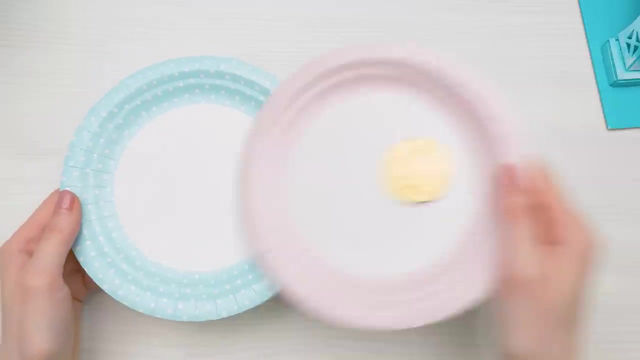 Then here's a plate for you, Even two Empty. Well, I'll put a chocolate coin here. Oh, Come here chocolate. Come to Papa. Why? Where It's for the magic trick, Look 1. 2.. 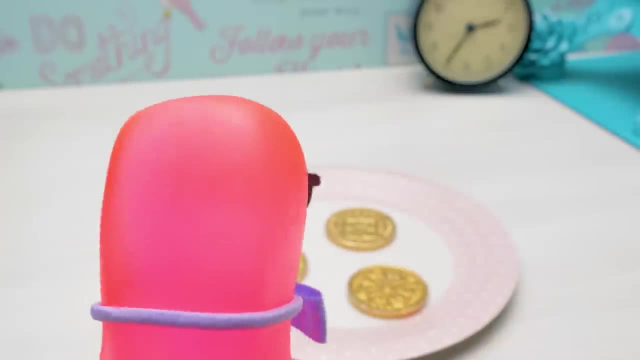 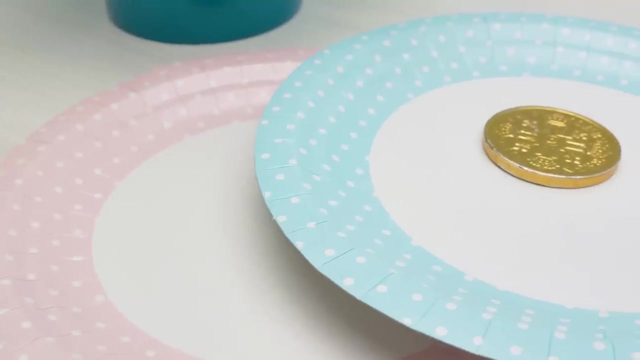 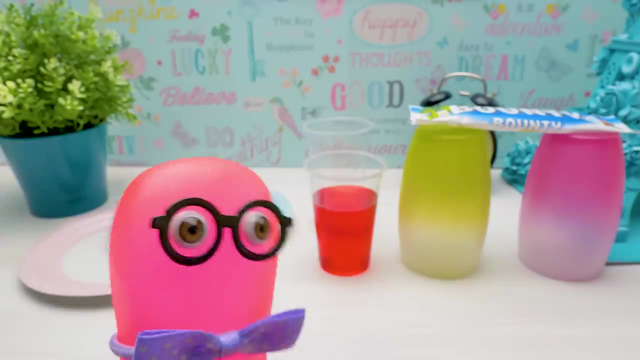 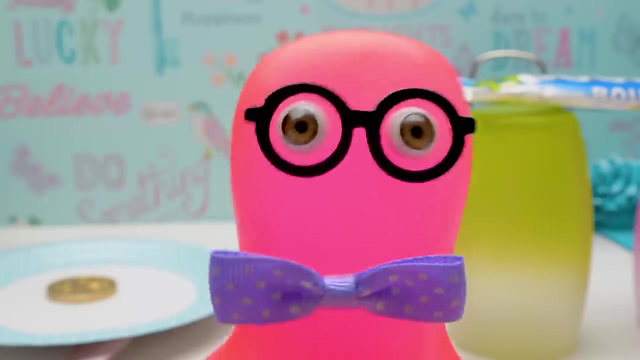 3!. Here you go, Chocolates out of thin air. I I even lost my appetite. I demand these secrets to be revealed, Right? so You're so impatient, Guys? do you want to learn the secrets? Of course they do. They've already subscribed to the channel and even hit the bell button, I'm sure. 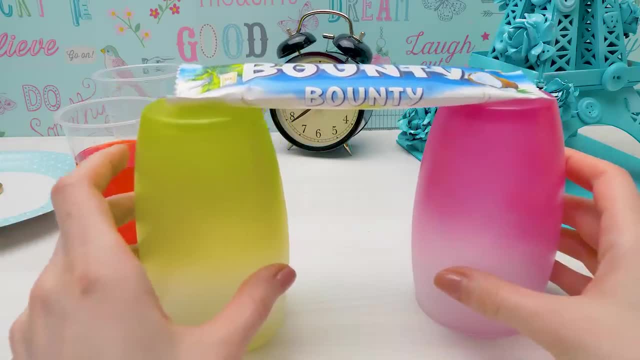 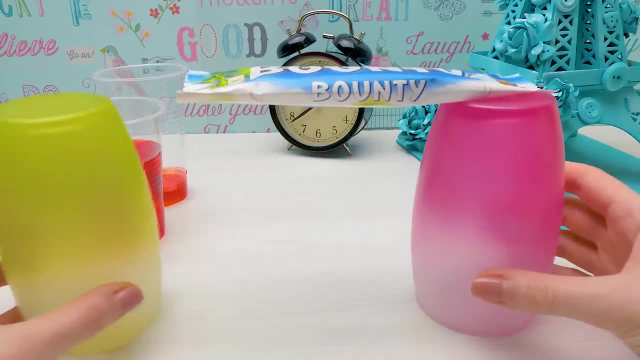 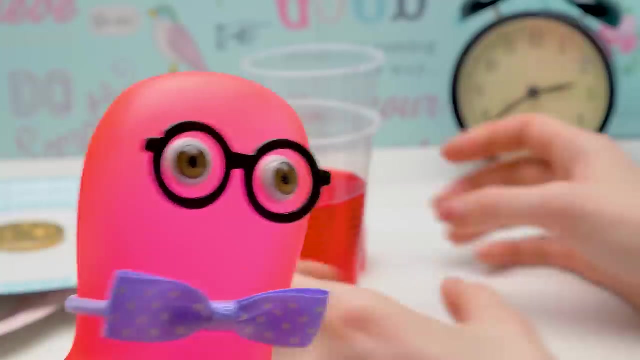 Well, alright for the first trick. In usual conditions the wrapper will fall, But what made it float in the air? There's a coin inside. That's why the wrapper doesn't fall Clever And the cup had a double bottom. There was juice in there. 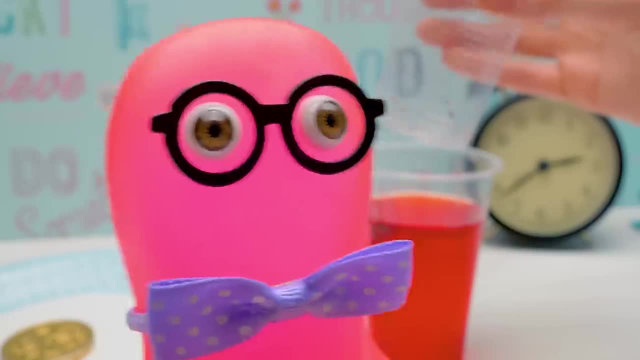 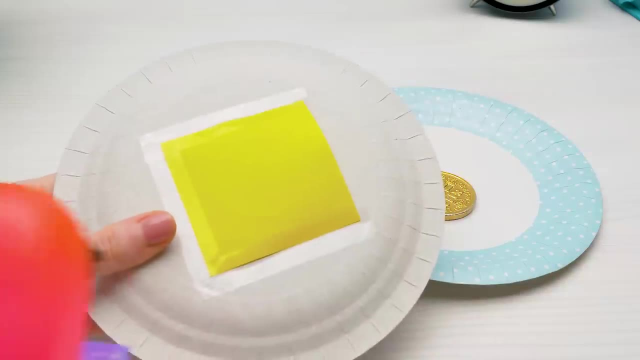 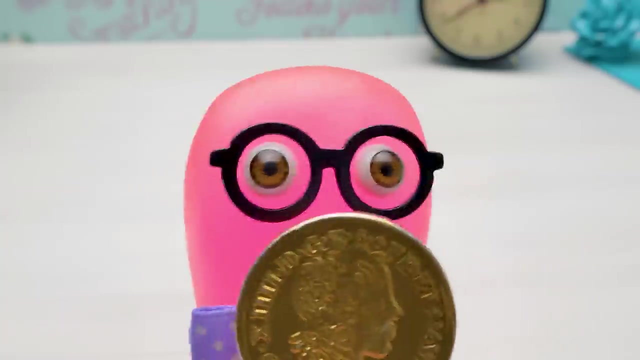 And the bottom just fell into the juice. Yep, That's why you didn't let me drink the juice. Good, I could have chosen. And as for the plates Here, Pockets, These plates know how to store stuff. Phew, The secret's been revealed. I can eat now. 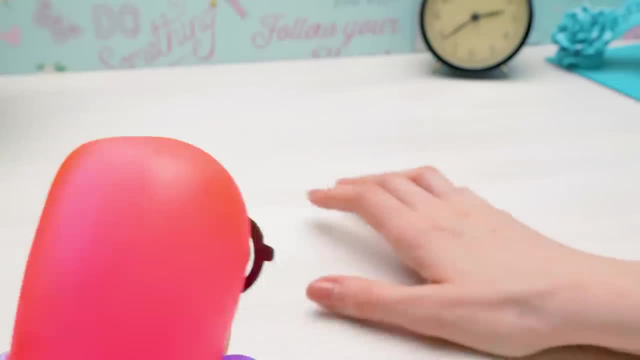 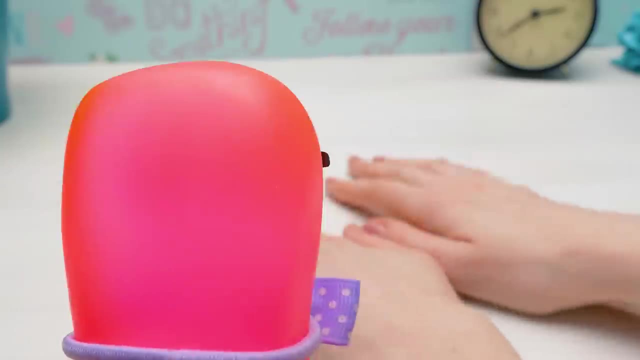 Hey, Sammy, don't go just yet, But Chocolates, Your chocolates, can wait. I have one more magical trick in store. Another trick, Which one? I can make a plastic bag with holes, not leak water. Come on, you can't do that. 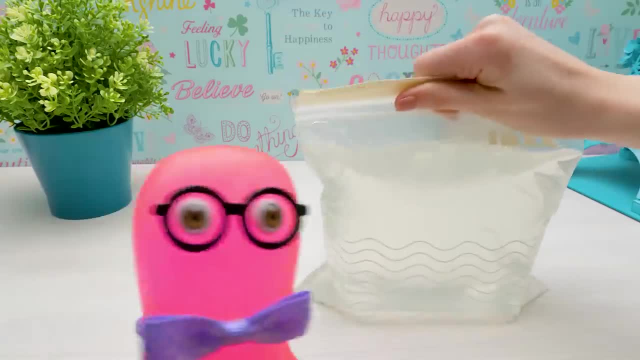 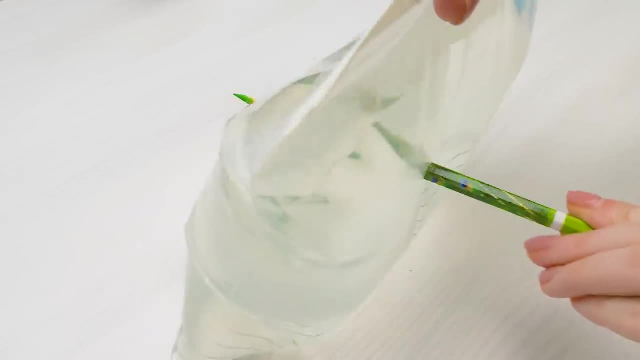 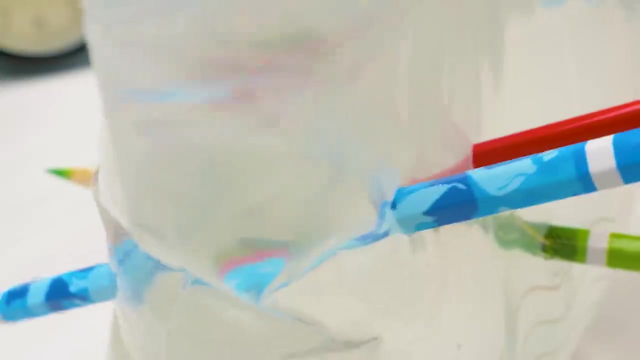 Oh, yes, I can. Here's a plastic bag with water. Uh, I'll watch here under the umbrella, just in case I'll take a pencil And Poke the bag through. Ha-ha, Water doesn't leak. And some more. 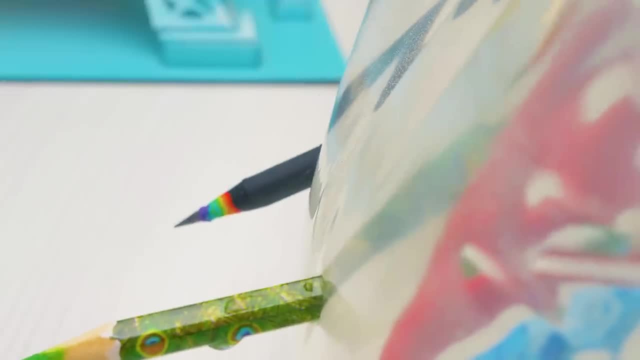 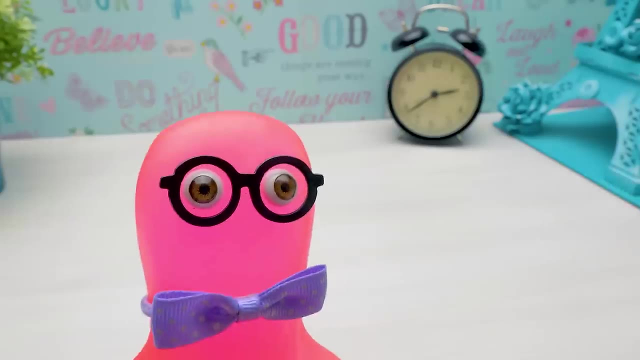 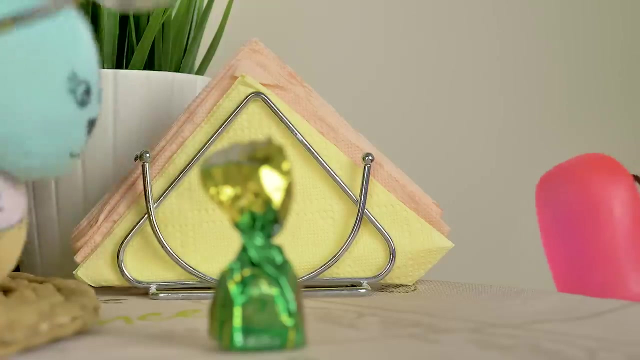 Oh Ha, Wh-wh-what, How, Why, It's the magic of physics, Sammy, Bye-bye. Hey guys, Did you like these tricks? Give a thumbs up if you did, And let's get this video to 2,000 thumbs up to get more magic in our lives. 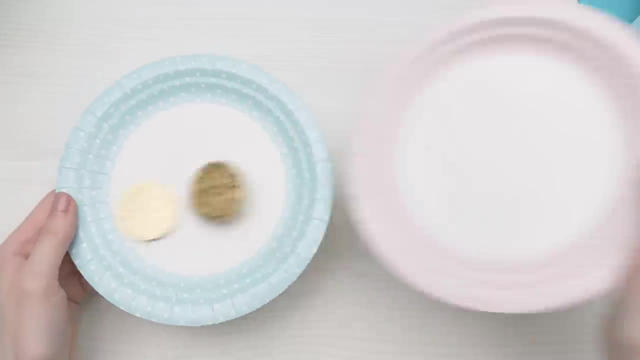 And Sammy and I will go think of something more magical.